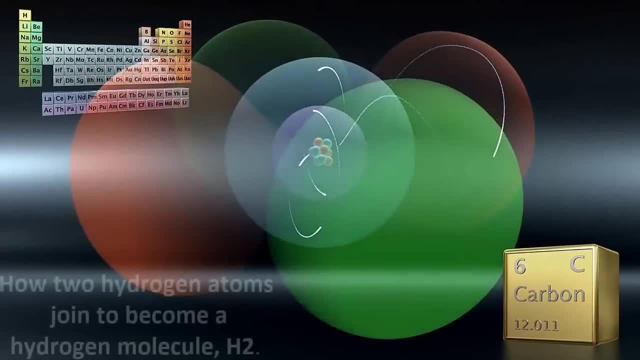 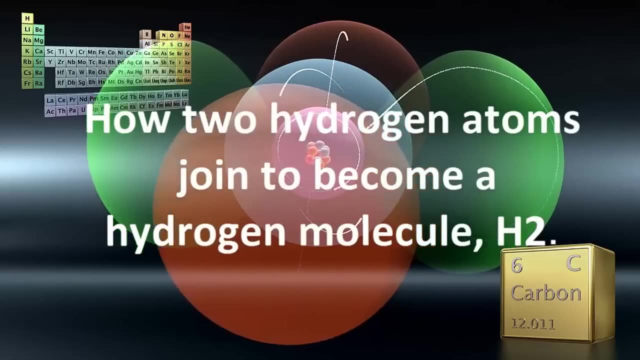 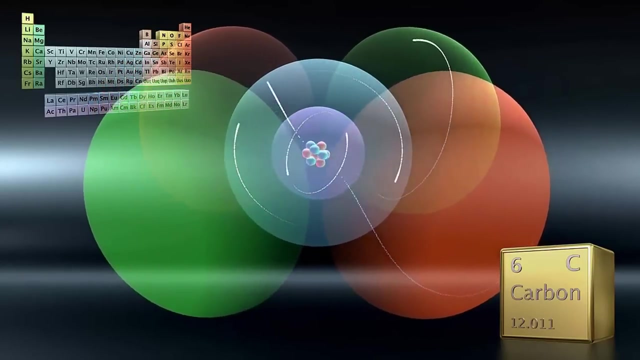 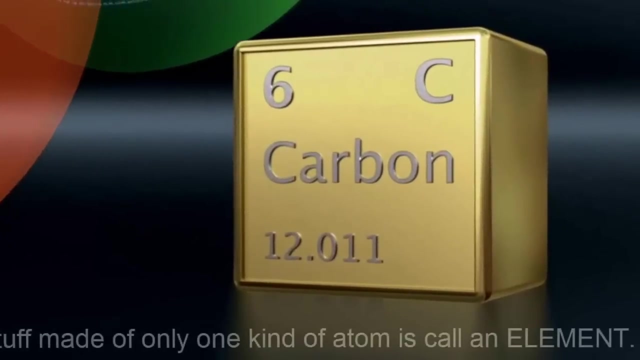 Remember we said that it's rare to find one kind of atom all on its own. True, it sometimes happens, and when it does we call that stuff an element Like the carbon in your pencil. But most atoms stick to other types of atoms somehow. 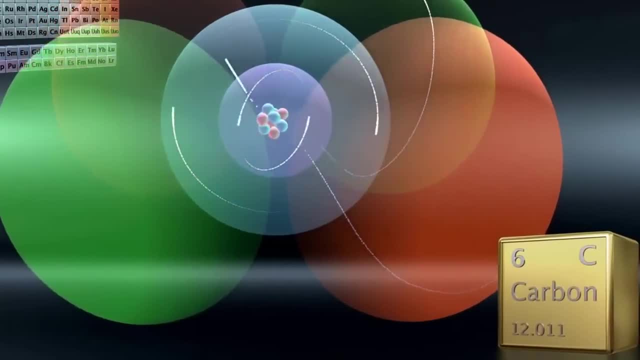 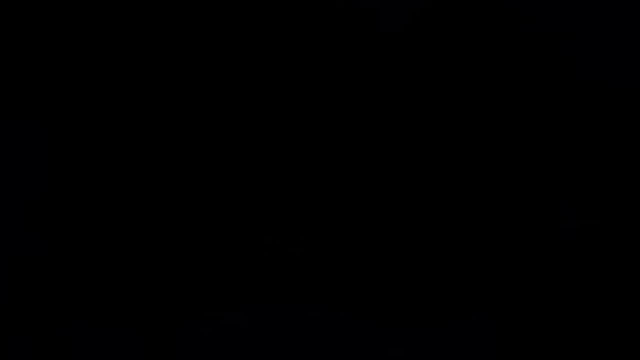 They usually like sticking to their own kind too. This video shows how they can do that. We'll start with the oldest and simplest kind of atom: hydrogen, made of one positively charged proton and one negatively charged electron. The electron moves amazingly fast around the nucleus. 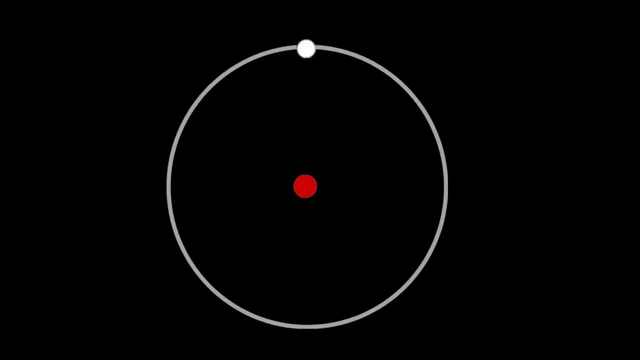 Why then doesn't it whizz off into space? Well, what kind of force would the electron and proton feel towards each other? Attraction or repulsion? I hope you said attraction, because they are oppositely charged. It's this force that bends them into moving in a circle around the proton. 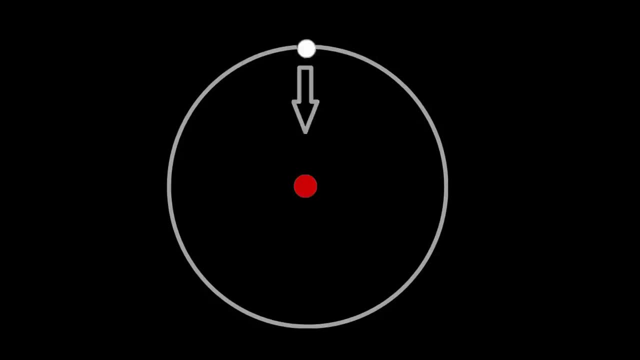 It's why atoms don't fall apart. Why don't atoms fall apart? Also, an atom is three-dimensional, Which means that the electron really whizzes around in the shape of a sphere, not a flat circle. Atoms are more like marbles than coins. 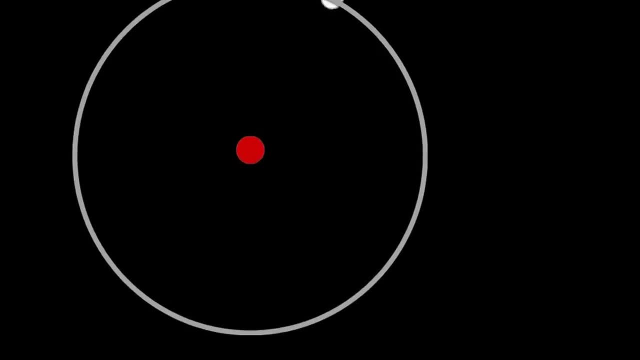 But here we will simplify the picture and show the electron in a circle and not moving. Now the main question we're asking is what happens when two hydrogen atoms come together. Let's bring another hydrogen atom onto the sphere, Let's see what happens. 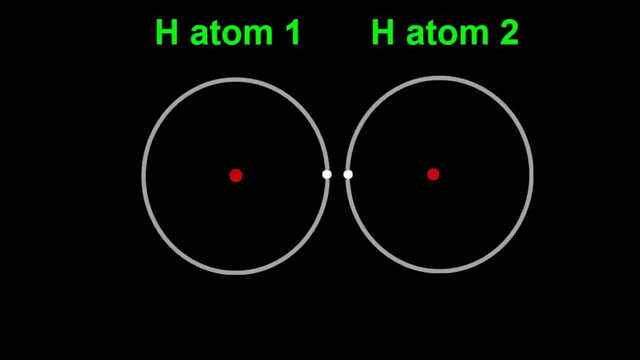 Will they bounce off each other and stay separate, Or stick together? Let's take a closer look at the electrons and protons. What happens when the electron from hydrogen atom 1 gets near the proton of hydrogen atom 2? Electron 1 and proton 2 don't care if they belong to different atoms. 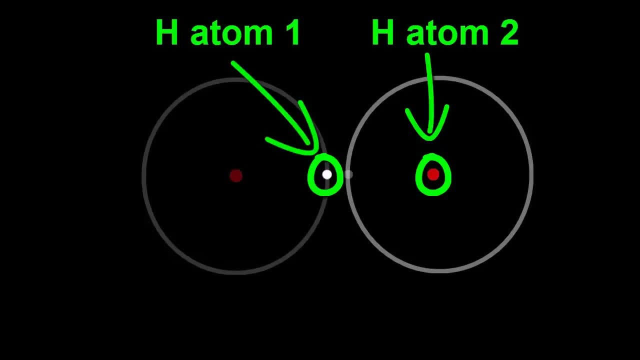 They will still be attracted. And here's the thing. The shell of atom 2 is not full. It can take up to two electrons. It has the space to allow the electron from atom 1 to visit it. The same deal happens between the electron from atom 2 and the proton from atom 1.. 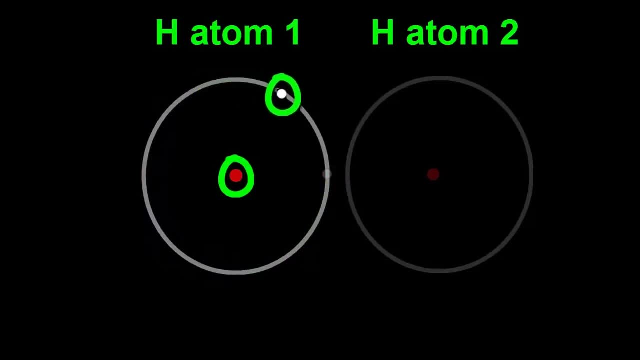 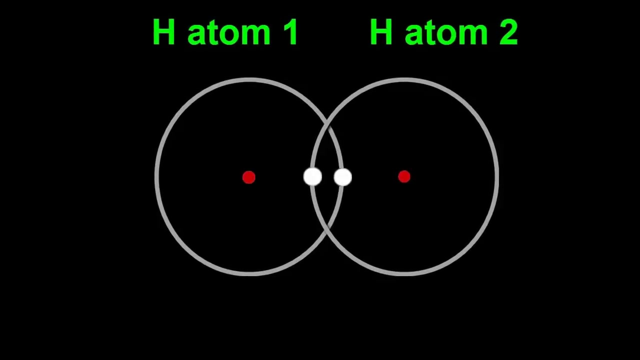 This means that both electrons wrap themselves around both atoms And they act as a kind of glue to hold them together. The two atoms become one molecule Because the shells are partially empty. they can overlap and merge, And the shared electrons then spend more of their time between the two nuclei. 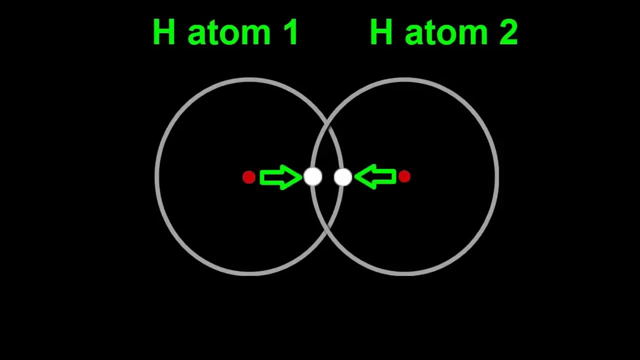 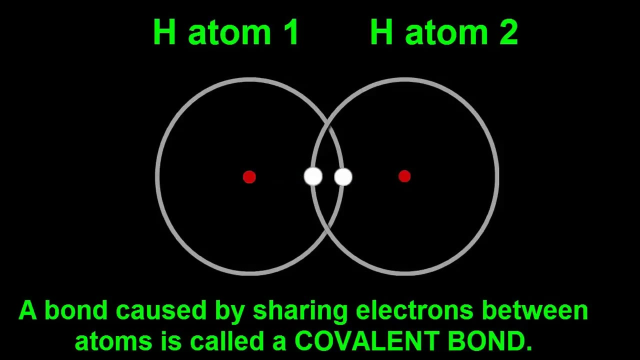 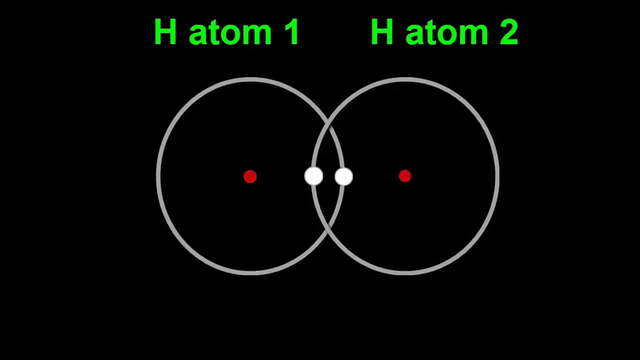 Because the nuclei are both attracted to both electrons between them, the atoms stick together as a stable molecule. This joining, caused by atoms sharing their electrons, is called a covalent bond. Is there a shorthand way of writing a hydrogen molecule? Scientists sometimes write a covalent bond as a stick between the two atoms. 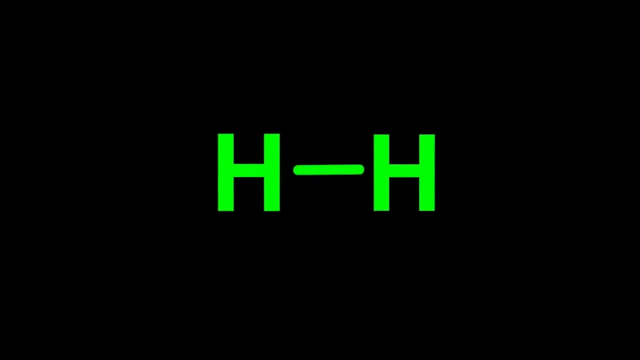 to show that they are joined. This way of writing is called a structural formula. They could show it even more simply as HH, to show that the two hydrogen atoms move around in pairs. Even simpler, they could write it as H2.. With the 2 standing for the number of hydrogen atoms joined by the bond. 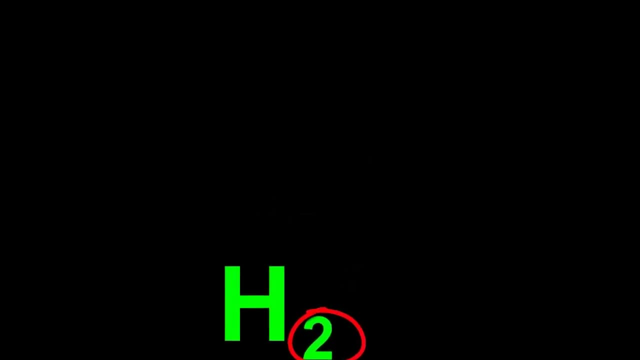 The 2 is written as a subscript. That is a little 2, a bit below the hydrogen symbol. This way of writing a hydrogen molecule is called a molecular formula Or just formula. Now let's see if helium can bond with itself like hydrogen can.